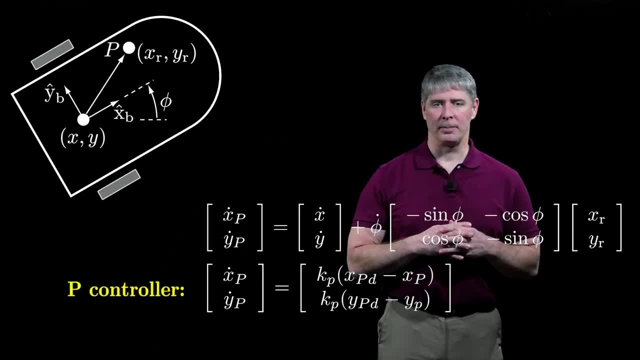 a desired trajectory, we could use a proportional controller which says that the velocity of the point is proportional to the position error. The commanded velocity of the point- xp, dot, yp, dot- can be converted to the linear velocity v and the angular velocity omega of the chassis Note. 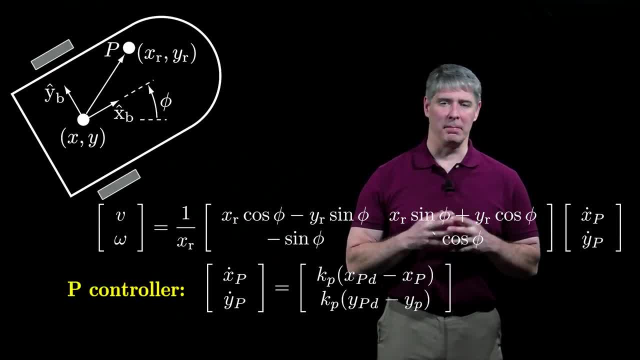 that xr- the x position of the point P in the body frame- must be non-zero to be able to move the point P in arbitrary linear directions. The constraints on v and omega depend on whether the robot is a unicycle, DiffDrive or car. 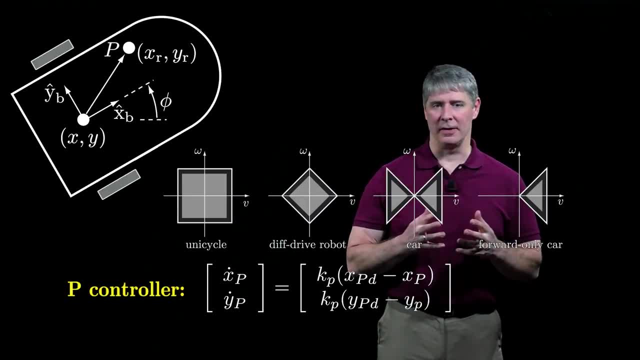 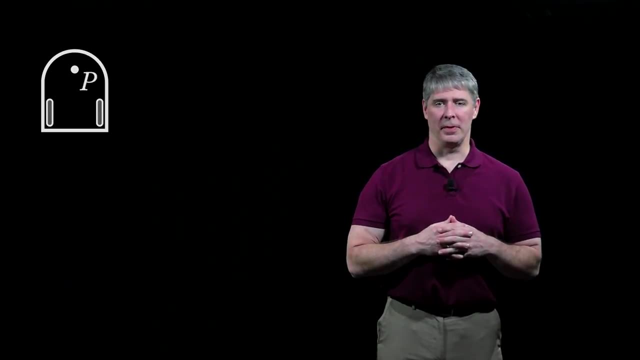 When initially planning the trajectory, the planner should use only a subset of the possible controls, such as those shown here. By doing so, the feedback controller has some extra control authority to make corrections to errors in trajectory tracking. Assuming a point P on the midline of the robot, this is an example straight-ahead trajectory. 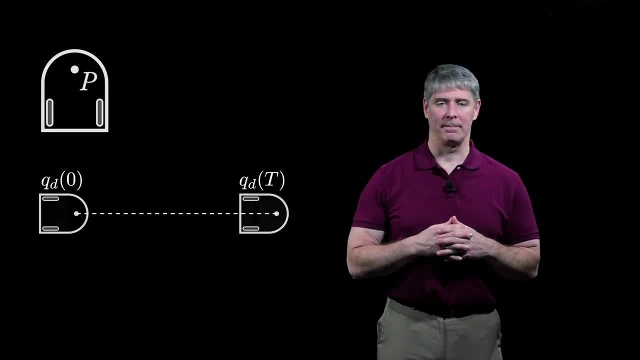 of the chassis and the corresponding trajectory followed by the point P. At any given point on the trajectory, the robot can satisfy the desired location of P with different orientations of the chassis, but only one of the orientations shown is consistent with the path before and. 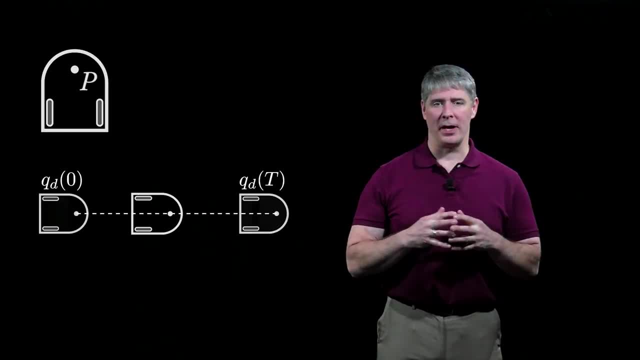 after this point. Therefore, even though the robot only follows the trajectory of the point P, this motion will often tend to align the robot's orientation to the desired orientation. For example, if this is the initial configuration of the robot, then proportional control of. 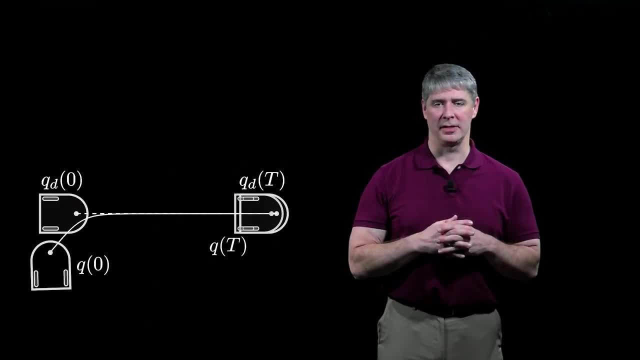 the point P will drive the full configuration of the robot to the desired trajectory. Notice that the robot's final configuration is a little behind the desired configuration. To reduce that error, we could add an integral term or a feed-forward term, as discussed by the robot. 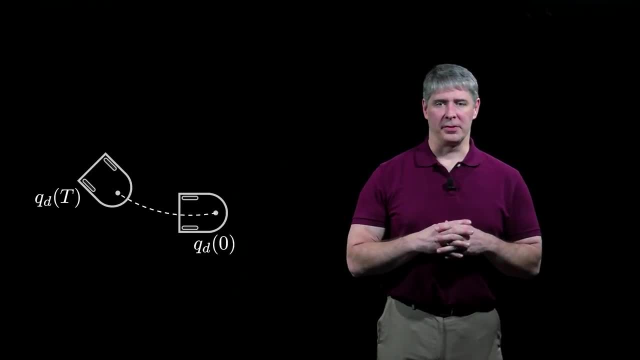 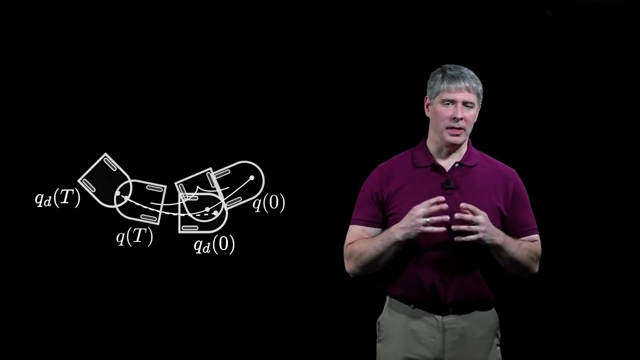 in chapter 11.. Here's another plan trajectory and the actual initial configuration of the robot. Proportional control of the point P causes the point to converge toward the plan trajectory, but the controller causes the robot to execute a direction reversal. So, even though the point P converges to the desired trajectory, the final orientation of 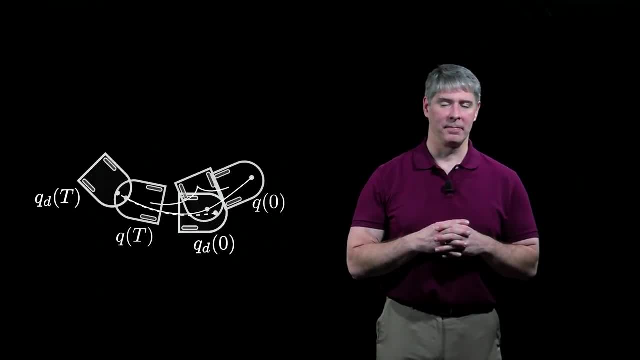 the chassis is off by nearly 180 degrees. In other words, just tracking the plan trajectory of a point P does not always result in good tracking of the full chassis trajectory. To track the full configuration of the chassis, we define the configuration of the frame B.